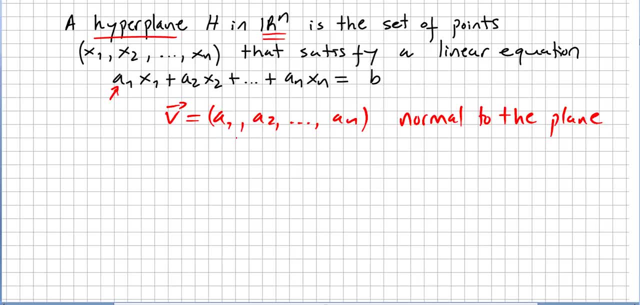 plane. Okay, so this, this is this. here are the components of the normal vector to the plane. So if you have a vector here, let's call this sorry. if you have a plane here, let's call it beta, or something like that. 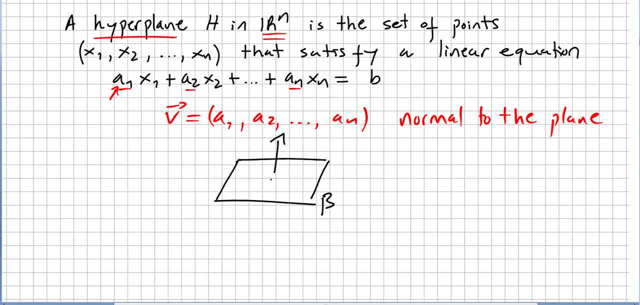 Okay, And if the equation of your plane is, let us say, x plus y plus b Plus z equals 2.. This vector, the normal vector to the plane, this vector here will be vector. so 1,, 1,, 1, right. 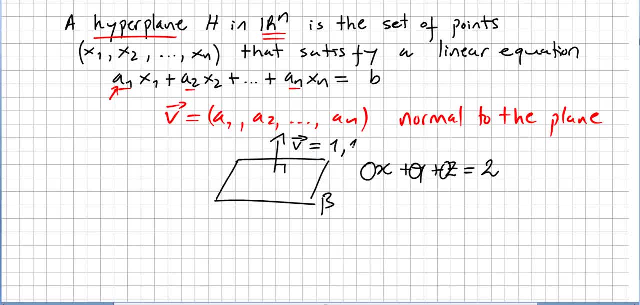 a1,, a2, an. So this will be vector 1,, 1,, 1.. So this vector will be normal to the plane beta. Okay, If you have. if the equation of plane is 2x plus 3x. 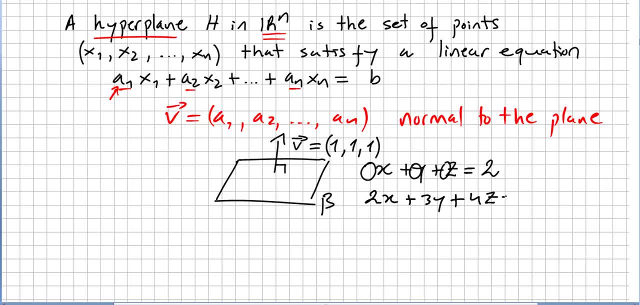 x plus 3y plus 4z equals 5.. The the vector, the normal vector for to this plane will be 2,, 3, 4.. Okay, Well, why is this a normal? Because any two points that you pick here in the plane. 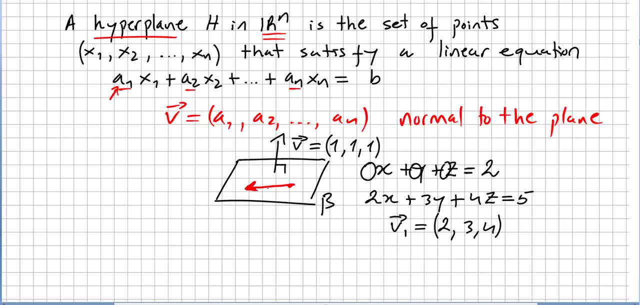 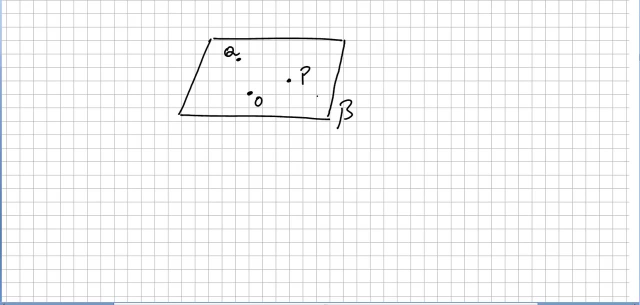 And if you take a vector between these two points, This vector here will be orthogonal to this, to any vector in the plane. Okay, let us say we have a plane here. Okay, So this is the hyperplane, Right. 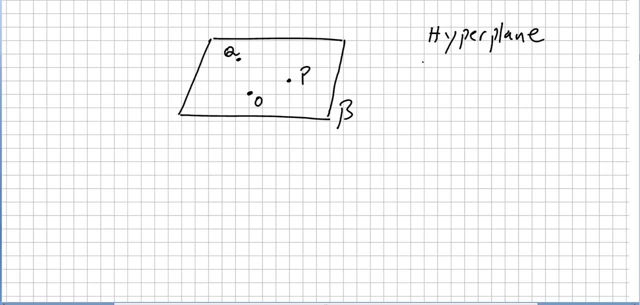 Just check the beginning of the video And let us say we have these points P and Q, So this point, this is point P, This is point Q And, of course, and O. That is going to be the origin here for us. 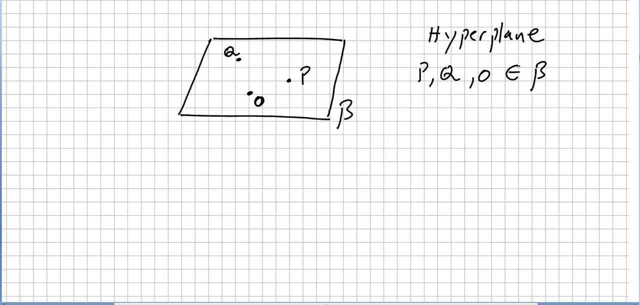 In the hyperplane. Okay, So we can take O P Right And let us call O P U, for instance, And we can take another vector here, Vector O Q. Okay, Let us call it something else, like W. 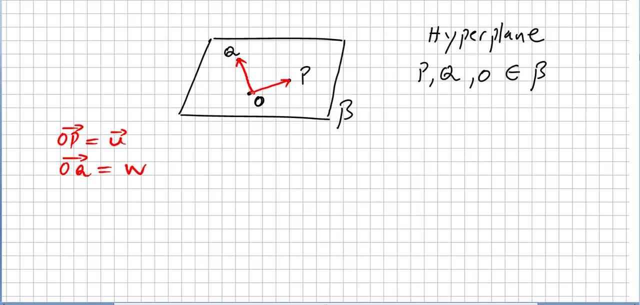 Okay. So O P is taking us from here to here, O Q is taking us from here to here. Right, And we can do now. So O Q is W And O P is U. Okay, So let us do W minus U. 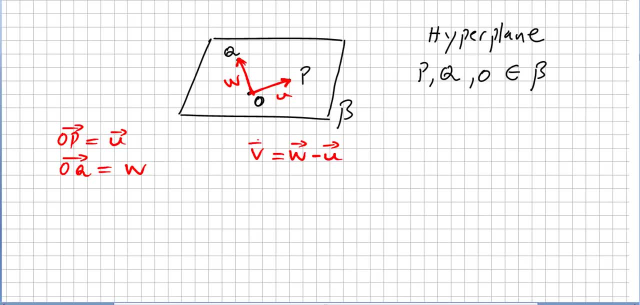 Okay, W minus U. Let us call this vector V. So W minus U, That will be this vector right. So this will be vector V Right, Because it is W minus U. Okay, So at the end of the day, what we have here is P Q. 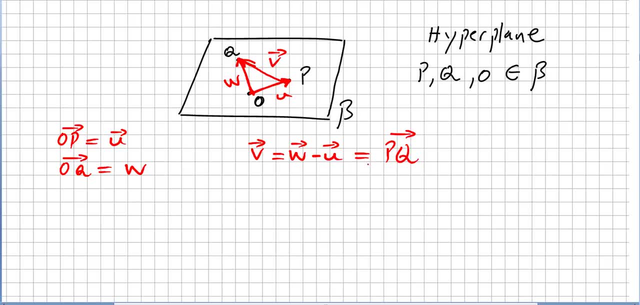 Right, We have vector P Q here, Okay, Okay, But the hyperplane will satisfy a given linear equation. Okay, And do not forget that we saw that the vector with components A 1, A 2, A n is the normal vector to the hyperplane. 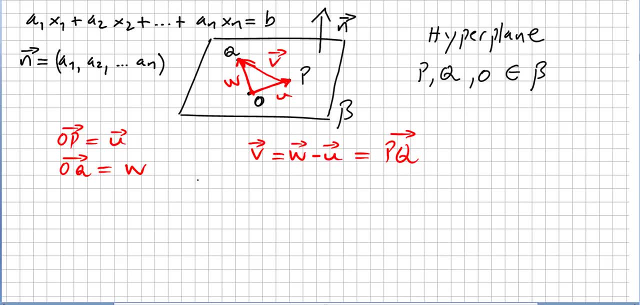 Okay, So one: if I take this A 1, A 2, A n, this normal vector, and I do it, the direct product, with U, vector U, I have to get B Right. And if I do the same,